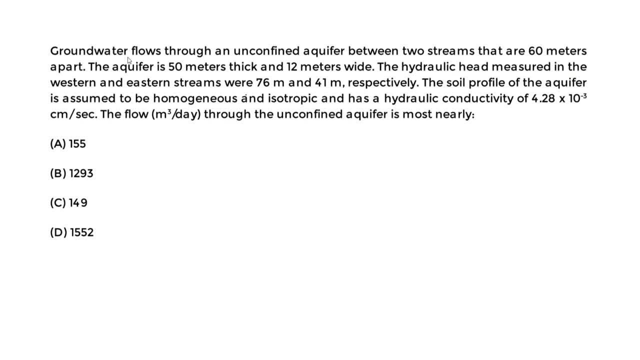 The hydraulic head measured in the western and eastern streams were 76 meters and 41 meters respectively. The soil profile of the aquifer is assumed to be homogeneous and isotropic and has a hydraulic conductivity of 4.28 times 10 to the negative 3 centimeters per second. 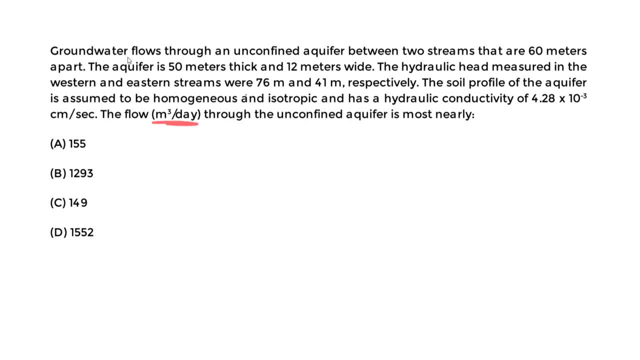 The flow in cubic meters per day through the unconfined aquifer. The aquifer is most narrowly what We want to find: the flow in cubic meters per day. So let's begin writing what we're given. We have to visualize what's happening, right. 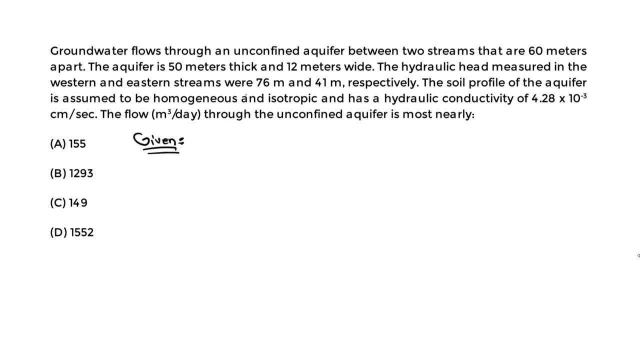 So they do this. They give you just a paragraph and you have to know what's actually happening. right, You have to have a picture and I recommend just draw whatever you can draw on the FE and make it like a quick sketch, right? 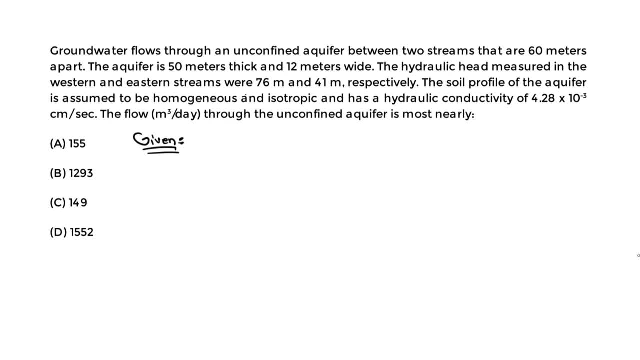 And you should practice that when you do a bunch of these examples. So the way I did this was essentially draw the aquifer first. So I drew the aquifer, So I drew the aquifer, So let's say we have the aquifer. 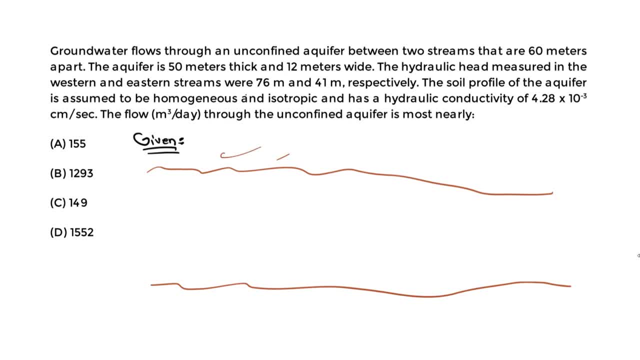 It's like below the ground right, Below the top ground surface, Let's say the top here is the top ground surface And we have a stream right. So what I denote it as we have the upgrading stream which is on the west right. 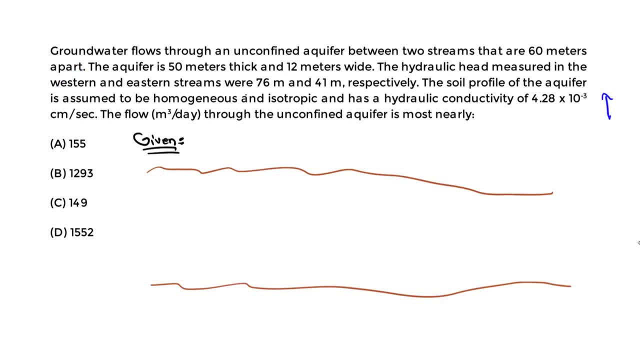 The west is this way. right, We know- let me label- that North is up, West is this way, East is this way, And we know south is this way. But we're looking at the west, So the western stream is going to be. 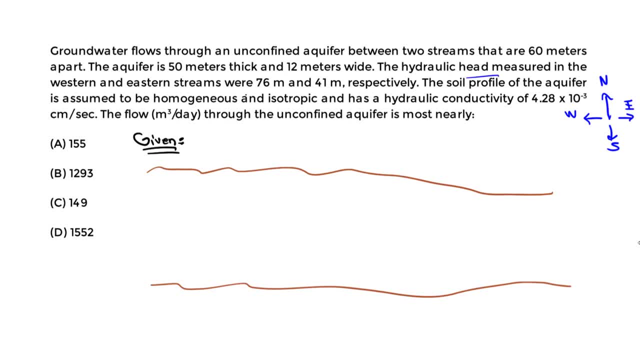 What It's going to be: 76 meters, And that's the head elevation from the bottom. So what we will say is: draw a stream here. This is the western stream. It will have a head elevation of a value of what It's the head elevation to the top water surface of the stream. 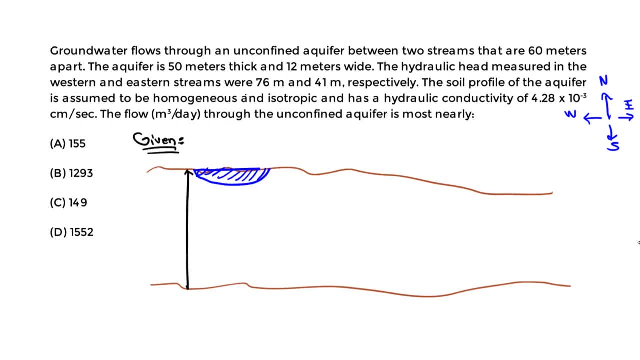 So the top water surface is always going to be just the top of the stream. So let me denote that here It's going to be the top of the stream Here. So we know that head elevation right to the top is 76 meters. 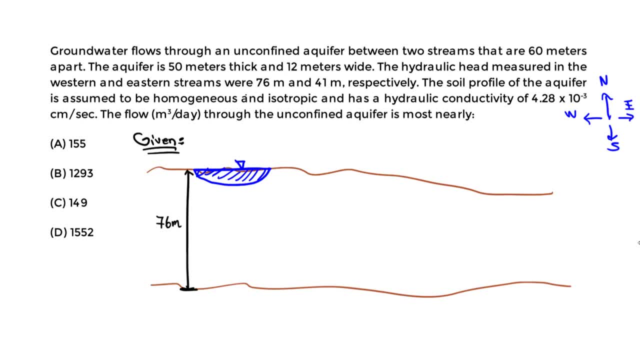 76 meters from the bottom. So we have that. Then we know that the eastern stream is 41 meters. So the way you read this sentence, the hydraulic head measured in the western and eastern streams 76.. 76 is for the western. 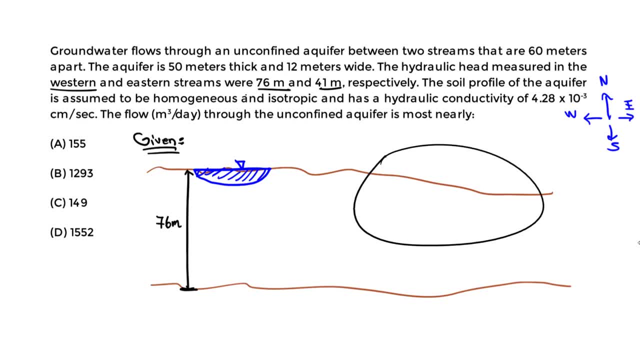 41 is for the eastern, right Eastern, So it's going to be the one on the right. So we draw that stream. It will have a top surface right And we know this is the eastern stream and it has the head is 41.. 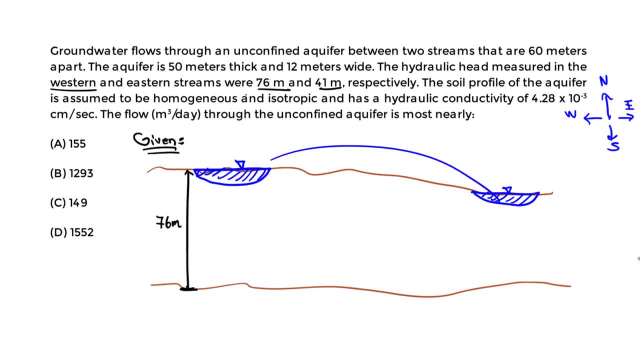 So it should be below 76. That's why I drew it below right. It's slightly below 76.. So that value, measured from the bottom to the top surface here, is going to be 41 meters. Okay, So we have that and we're told that the two streams are 60 meters long. 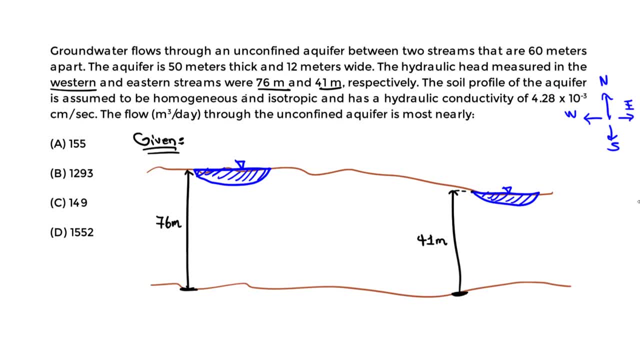 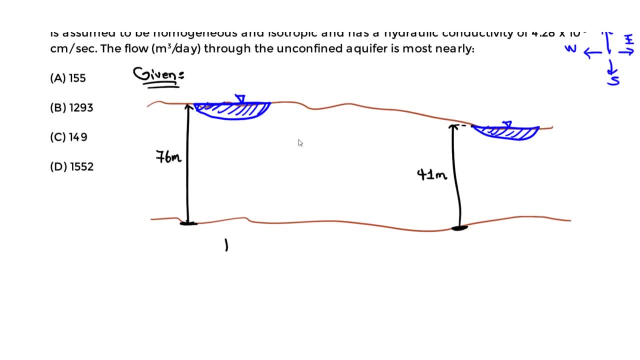 60 meters apart. So this is important- The two streams are 60 meters apart. Remember that's our dx right, That's the dx distance. So let me go the two streams here. the distance between them is going to be the delta x. 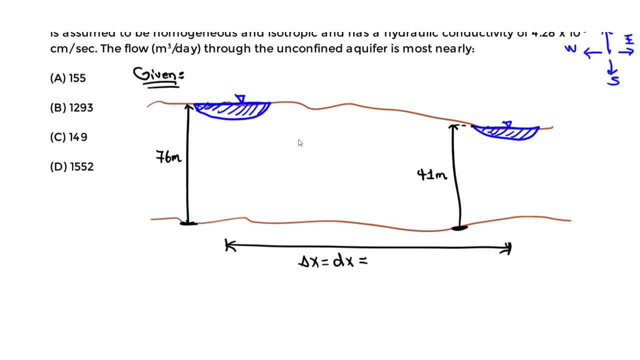 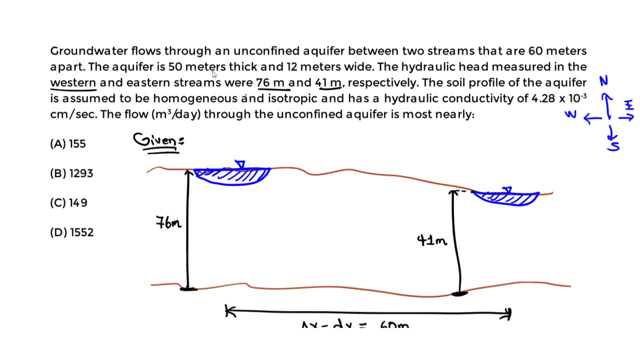 which is the dx, And that's going to be the 60, 60 meters. So we have that and we know that the aquifer is 50 meters thick And 12 meters thick, 12 meters wide. So you have to be careful with this. 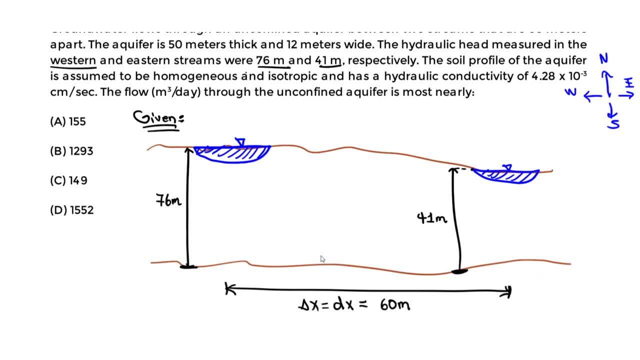 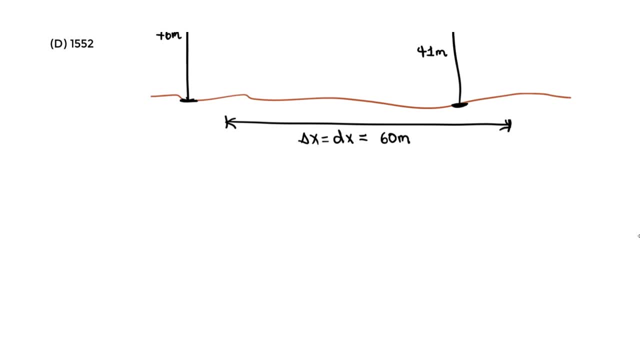 This view is a side view. right, It's a side view of the aquifer, But if I draw a, well, let's call it a perspective view or an isometric view of the aquifer or a 3D view. it looks something like this: 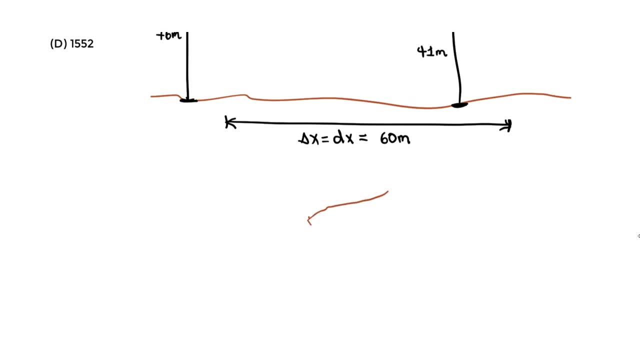 Let me actually draw it here. It looks something like that: We have the aquifer, We have this thing here, The aquifer, And it's below the ground surface right. Let's say, this is the top surface where we stand, right. 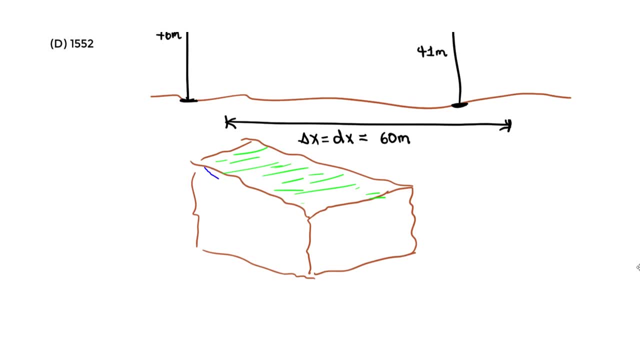 And we have the streams here, right, We have a stream here And this stream does something like that, And we have a lower stream here. right, This is the eastern one, A stream like that, And we know this aquifer. it has a width. 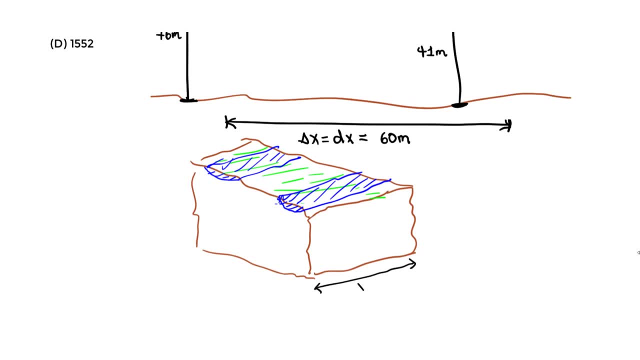 This is the width right, The width of the aquifer. We'll call it W And the thickness of it is going to be your Y. It's the thickness in terms of that Y distance. So the thickness of the aquifer is always this distance when you look at it in 3D right. 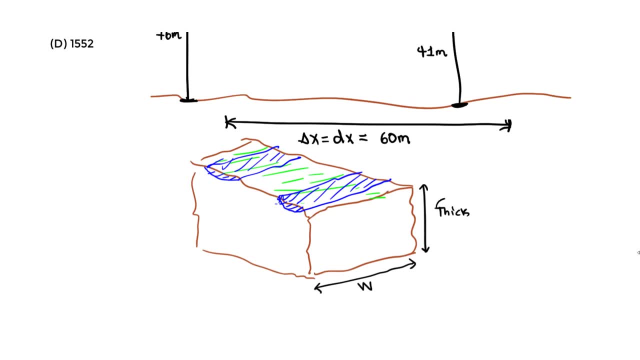 So that's the thickness. How thick is this aquifer? That's going to be that right And the thickness. we typically give that the B value And we'll see how that applies later, But the B value is the thickness. 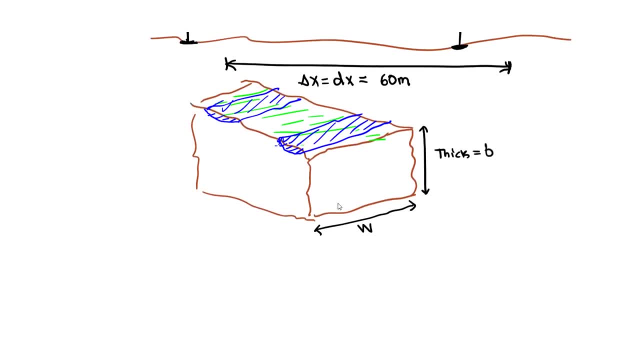 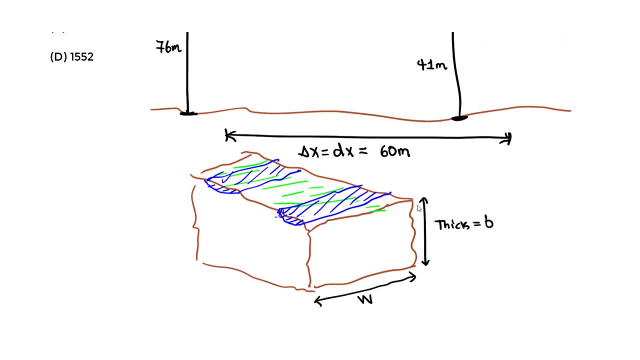 So just know, when you have an aquifer, if you look at it in like 3D, the width is like into the page. If you look at a side view, it's into the page And the thickness it's like your elevation, right. 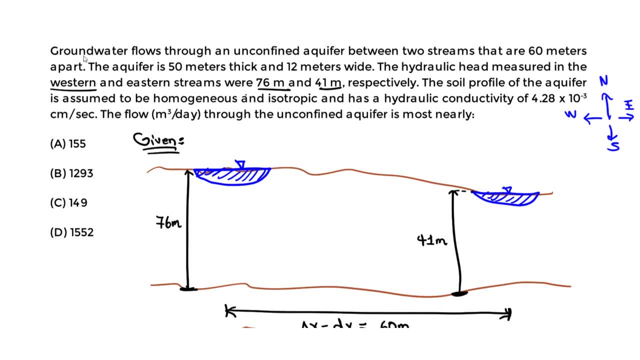 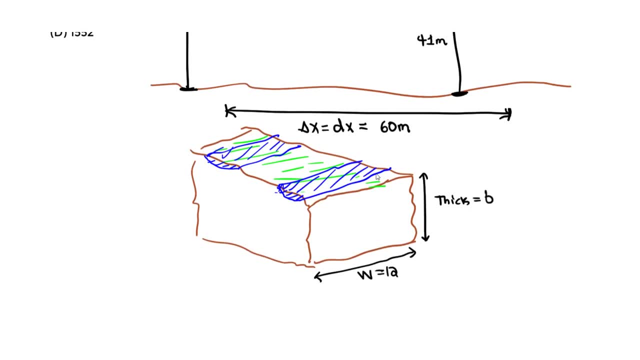 But we know we're told the thickness And that thickness is given to be how much? Fifty meters, And the width is twelve meters. So we'll label that The width is twelve meters, The thickness is fifty meters. Okay, So we need that because that allows us to find the area right. 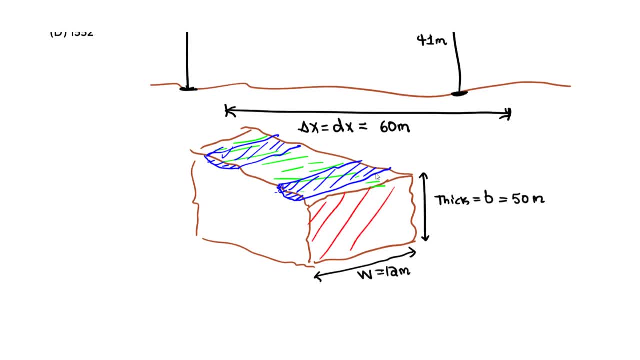 The cross-sectional area that the water flows through. It's essentially this area. That's the area we need when we use Darcy Law And that's the area we're always looking at. You multiply the width times the thickness. That's how you get the area. 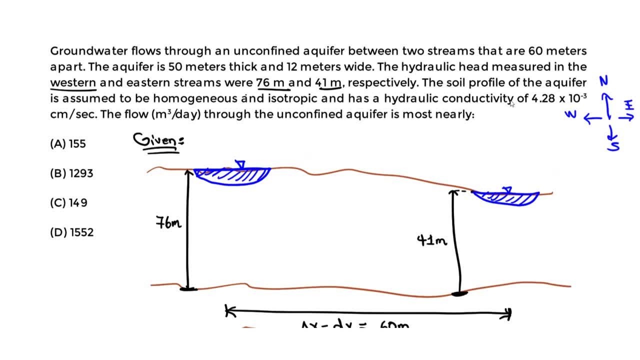 So we have that, And that's taking care of those two values And the hydraulic conductivity is just given. That's the K value, right? Okay? K is four point two, eight times ten to the negative three centimeter per second. So we have that. 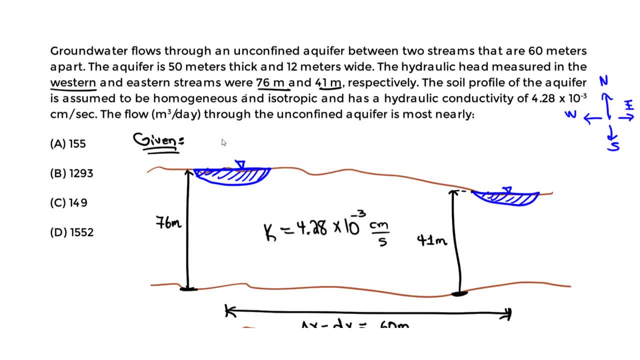 Now let's apply Darcy Law to find the flow. And why do I use Darcy Law? Why do I not use the Debut equation? Because we're not looking at the cone of depression. right, We're not looking at that cone of depression. 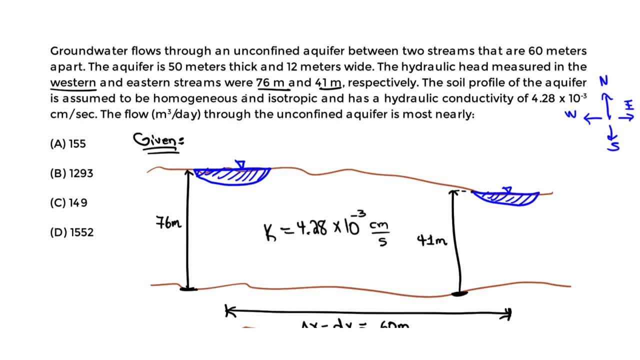 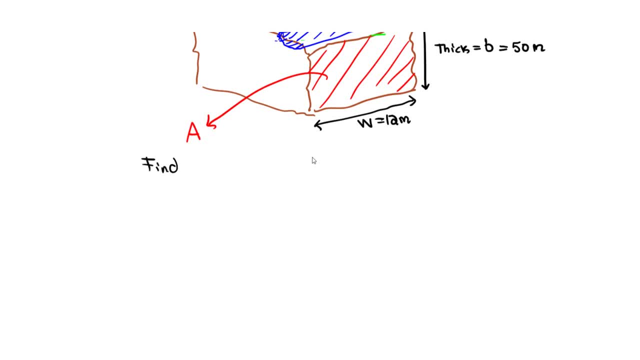 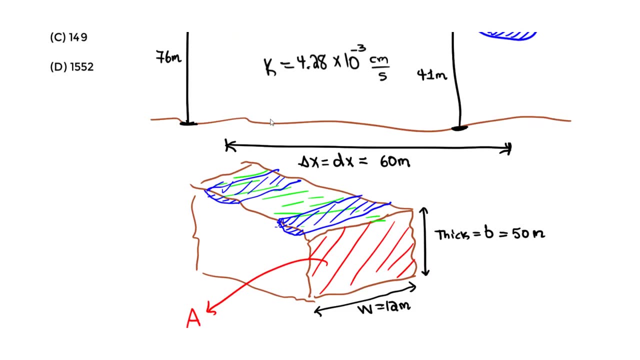 Or we're not asked to find draw down right. So what we will do is just apply Darcy Law. So we will use Darcy Law to find Q. And we want to find Q specifically in what units. it says in cubic meter per day. 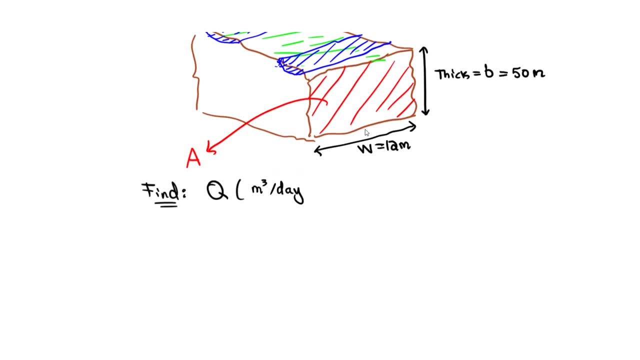 So we have to be careful with the units right. So doing that for the solution, I'll write the Darcy equation for us, Q equals negative K. A, dH over dx. This dH over dx Again. This is the hydraulic gradient. 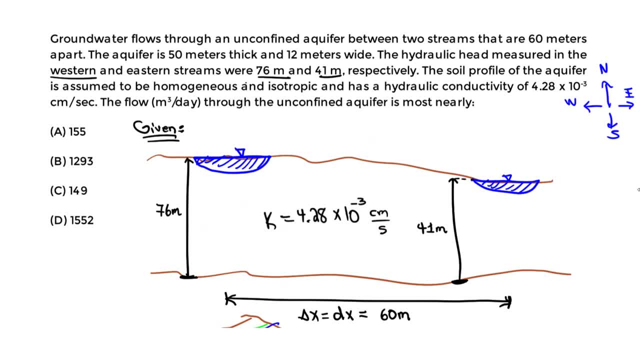 It's essentially the slope of the water table And in this case, the slope of the water table does something like this: We go from the up to the down. This is essentially the slope of the water table. This is the I right. 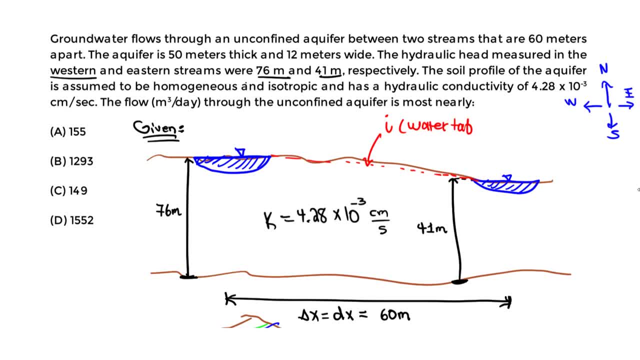 Where the water table is, at Water table. So we're actually like sloping down right. We're sloping negative if we draw it. This is the western eastern stream, So we slope negative. in that case. That's the direction water will travel. 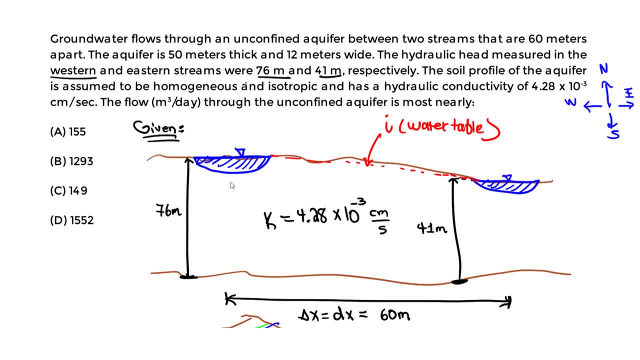 So water will travel from the top stream where the water table. So this is just an extra note. But if they ask a conceptual question, this water table here it's below, It's below the stream, right, But then when you, this water table has to be above the line here. 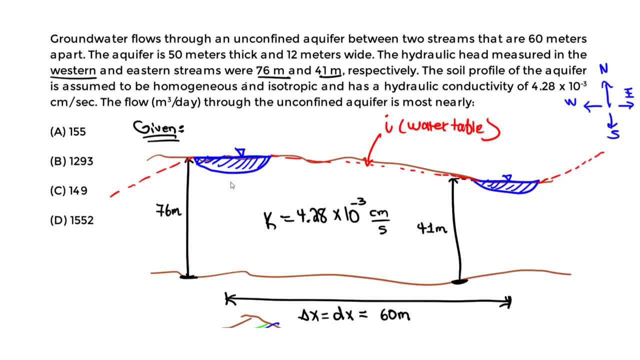 You see how this line is above the stream. That tells me when the water table. this is the water table line here. right, This is the water table. If the water table line is above the stream, this is the water table line. 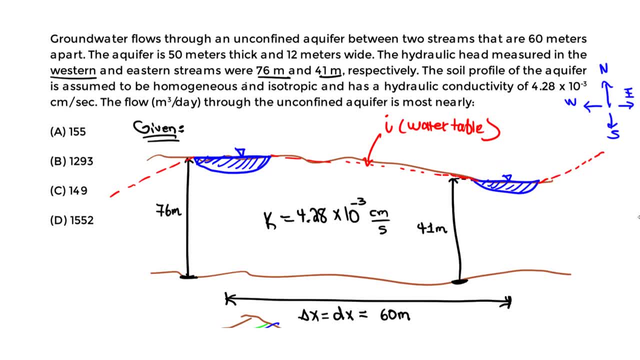 If the water table line is above the stream, water is going to travel into the stream, So water will try to flow this way. But now this is the opposite, right, The water table here. let me draw that. The water table here is below, right. 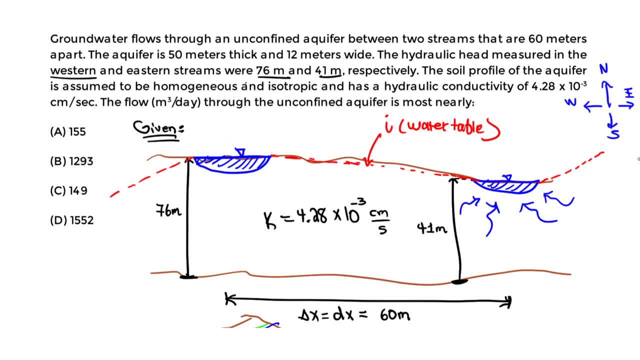 This line, the water table line, is below the stream, So where is water is going to leave? the stream, right, So it will leave. the stream It will leave, So that's important to know. right, Looking at that, When it's below, it leaves. 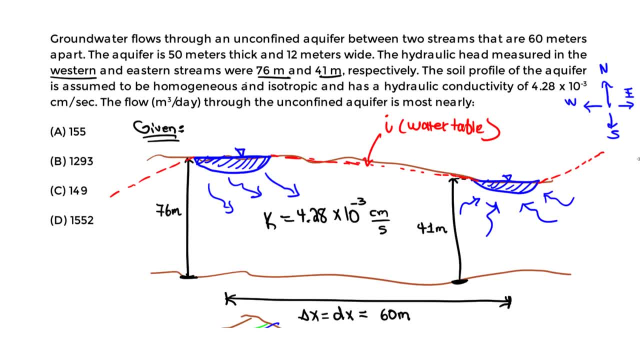 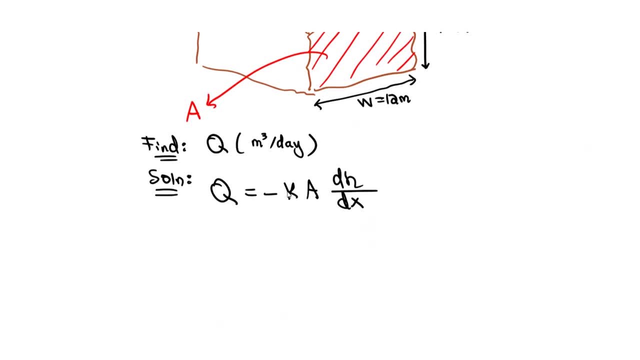 When it's above the stream, the water table line, it enters the stream. So here we're discharging water, Here we're adding. So that's just a note, Let's apply Darcy Law. Darcy Law, We know that we will first find the dH over dx. 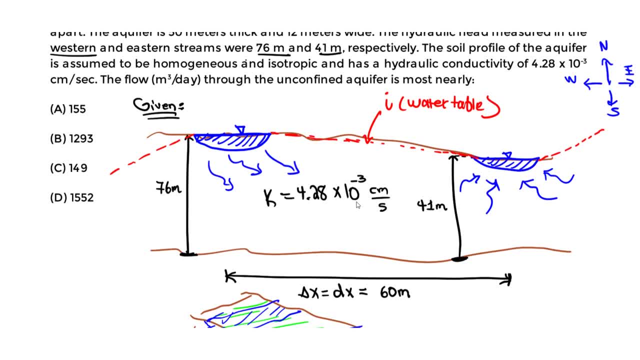 That's the hydraulic gradient. So the hydraulic gradient, in this case, we know that change- dH is your change in head, So dH is your change in head. So I go from the top surface of this, the western stream, to the surface of this. 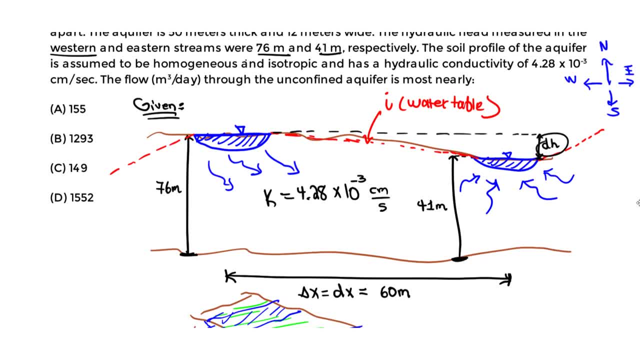 So that gives me my dH value. So how do you get the dH value? How do we get that? You just take 76 minus 41. And it gives you that dH value right. So dH is 76 over 41.. 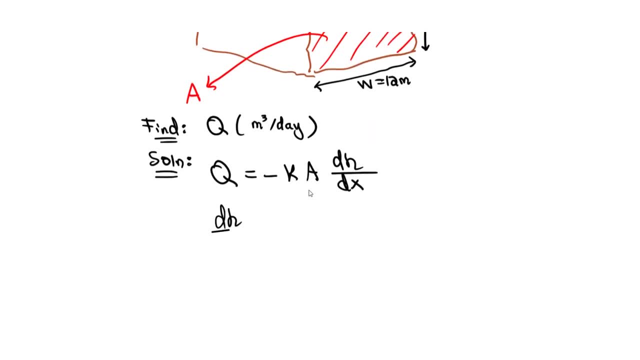 So what I'll do is even I won't plug it all in, so I'll just solve for it here and plug it in later. So you do the 76.. Minus 60 meters, minus 41 meters And divided by your dx. 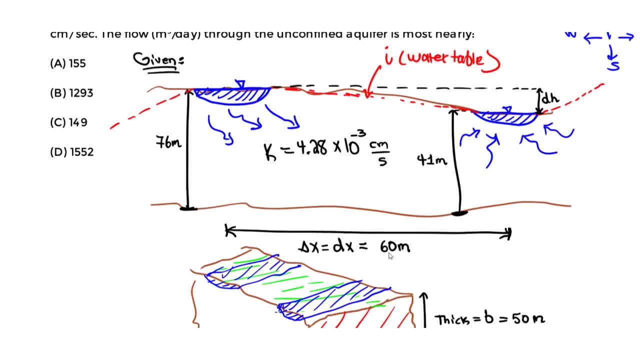 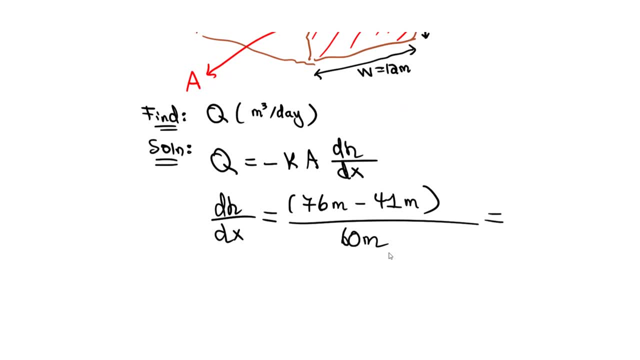 So what's the dx? dx is given to be 60, right, That's the dx, the distance between the streams. So that's 60 meters. So, doing that, you do the math there and you get your hydraulic gradient. We call that the. I value dH over dx. 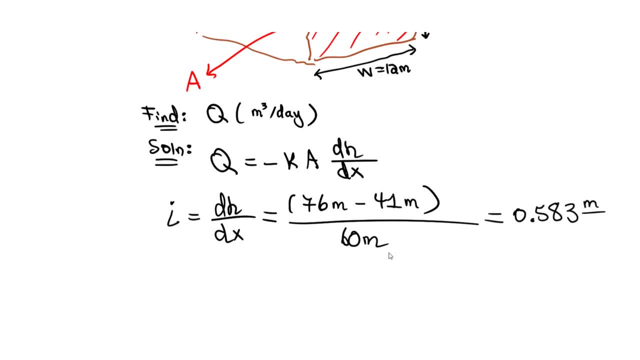 That's going to be 0.583 meter per meter, So it's a drop. It's a vertical of 1 meter per a horizontal distance traveled of 1 meter, So that's essentially your slope. So we know, in this case it's like a negative right. 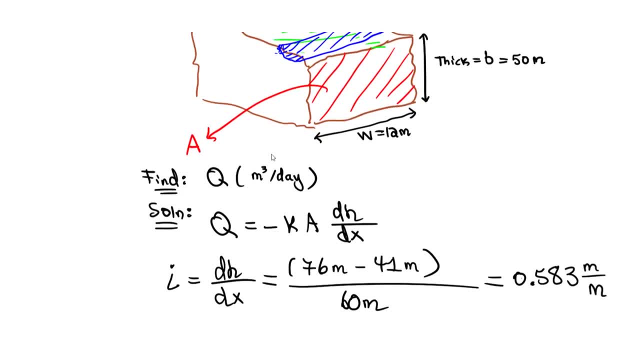 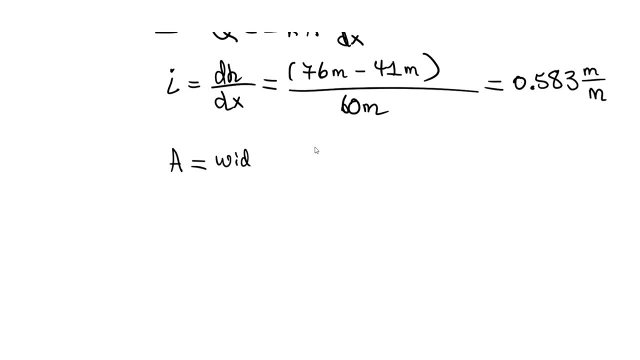 Because it goes down. So we'll just plug it into the equation. Then we do the area. The next step I'm going to find the area. We said the area is the width times the thickness, Always. So you have to know that. 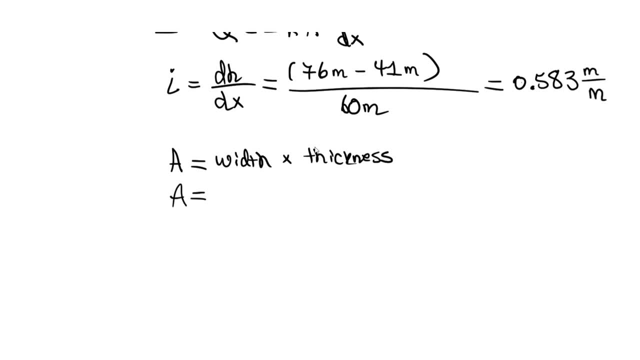 And we know the thickness. It's called the B value, so the thickness is the B value. let me just double check if that's correct, because we know the thickness is the B value because that applies when we use the time equation. but just know the thickness is always your B value and 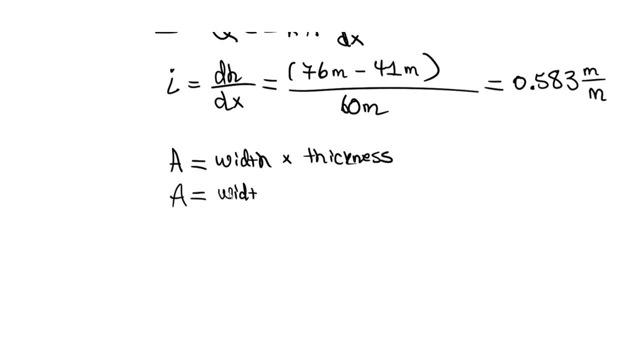 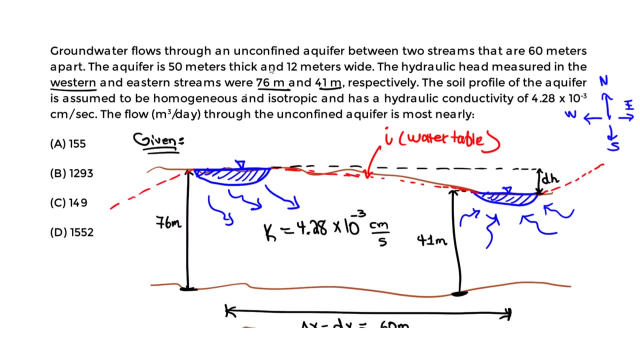 we'll see how that applies. so it can be the width times the B value, which is always the thickness. so what's the width in this case? the width is 12 meters, we're told in the problem, statements 12, and the thickness is 50 meters. so we 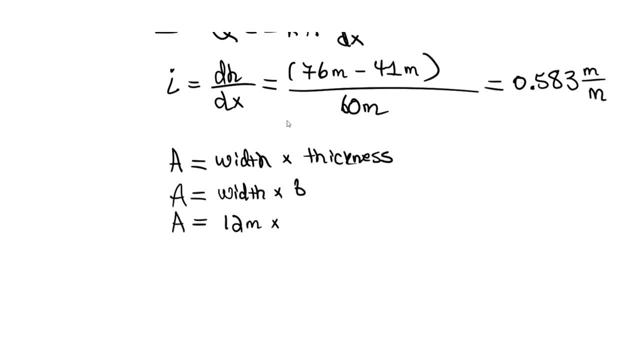 just do that right. so you do 12 meters times 50 meters and doing that, let me see what I get. you get 600 meter squared, so that's taken care of. then we solve for Q finally. so we solve for Q. we know the K value is 4.28, right? 4.28 times 10. 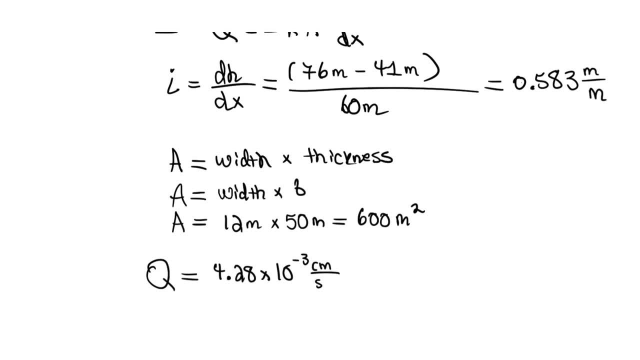 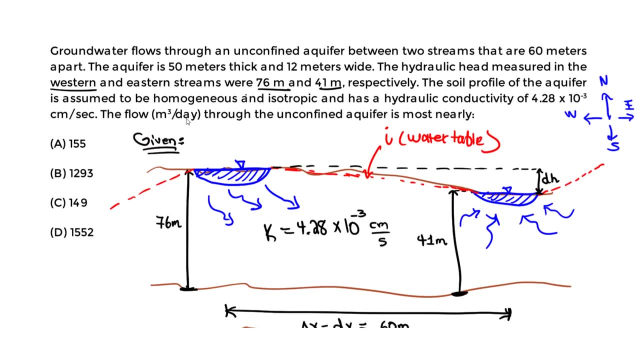 to the negative: 3 centimeters per second, centimeter per second. so now you have to be careful with the units. we want cubic meter per day, so we want to take out the centimeter and convert it to meter, and we want to take out the seconds and convert it to days. we have 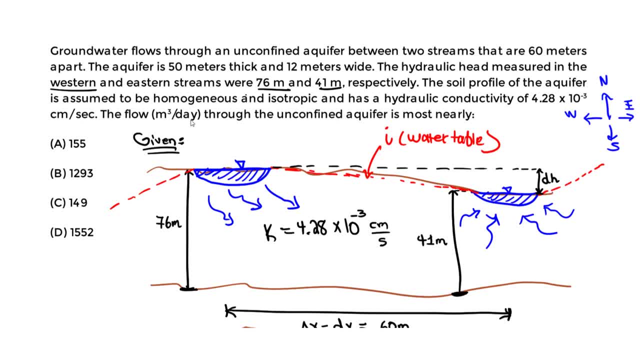 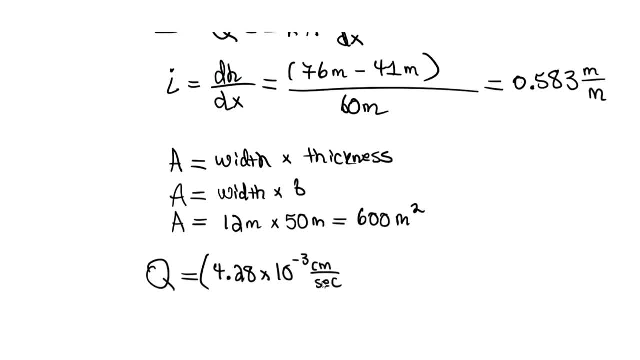 to, because we want cubic meter per day. we only want meter for the distance units and days for the time units. so I'm gonna convert this. I'll convert the K value and we know how many centimeters centimeters here we have to put centimeters here, how many centimeters are in one meter? 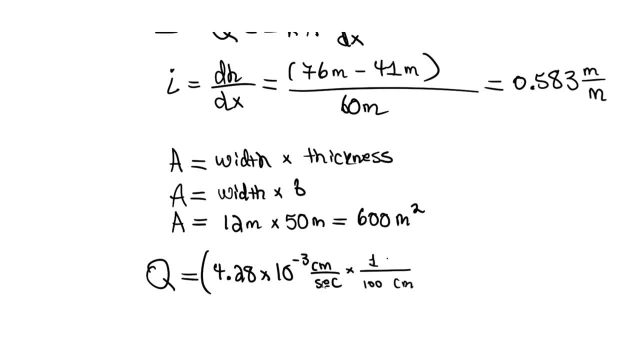 it's always a hundred centimeter in one meter. so these cancel. then, how many seconds are in a day, right? so this one is good to know how many seconds are in a day. there's eight thousand six hundred eight eighty six thousand four hundred seconds in one day, so that's always. that's a handy, a very handy one to know. 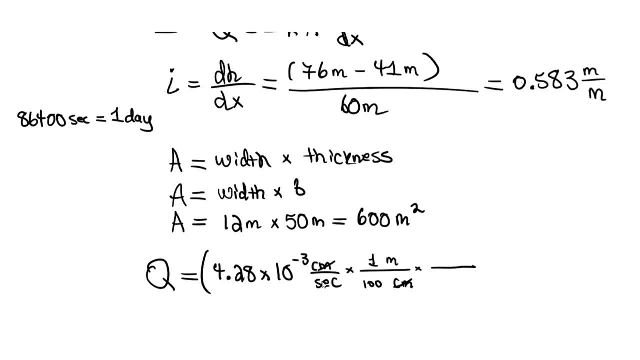 write down your equation sheet and know that. and there's another one to know: there's three thousand six hundred seconds in what in one hour? right in one hour. so that's also a good one to know that these are very common, right? so we know what we will do is see there's eight thousand six hundred eighty six. 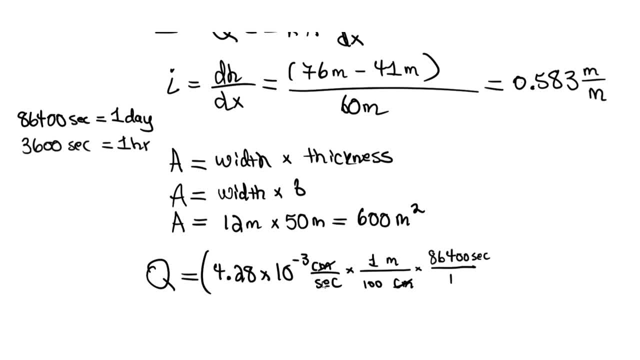 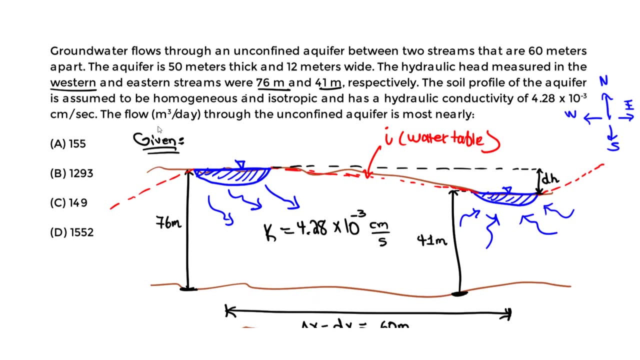 thousand four hundred seconds in one day. okay, so the seconds cancel and what we get is meter per day and that's what we want. that's correct. so this whole thing is actually the conversion. for what? for the K value, because I want it in meter per day, I want cubic meter per day thing. so I need 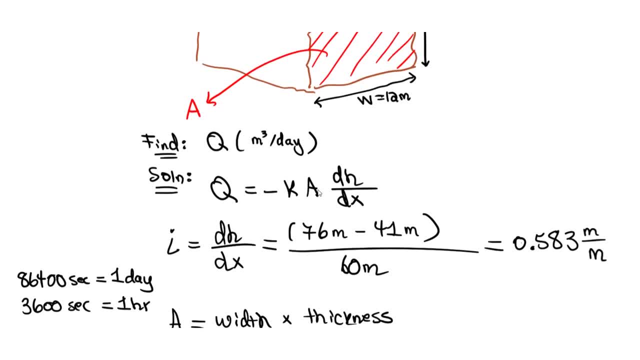 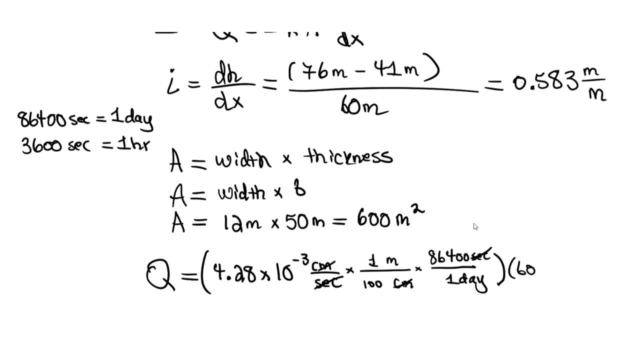 meter per day here, right, so we've taken care of that. then we multiply by a and multiply by dh over DX. so the a value we said is six hundred meter squared and we multiply by dh over DX the gradient which is the zero point. five, eight, three.